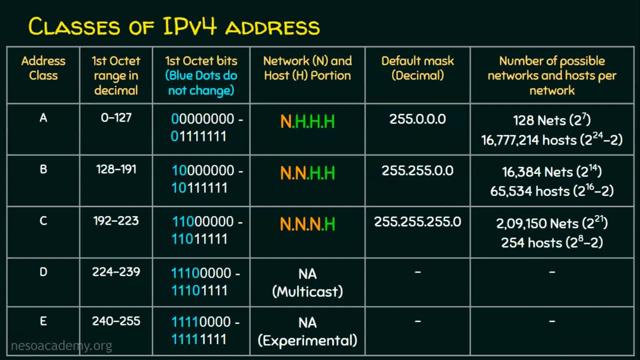 create a network with 200 devices, then we can obviously go for class C. Any class C network can cater up to 254 hosts, In case if our requirement is 300, so we can't go for class C Because in class C the maximum number of hosts or devices possible is 254 only In order to handle 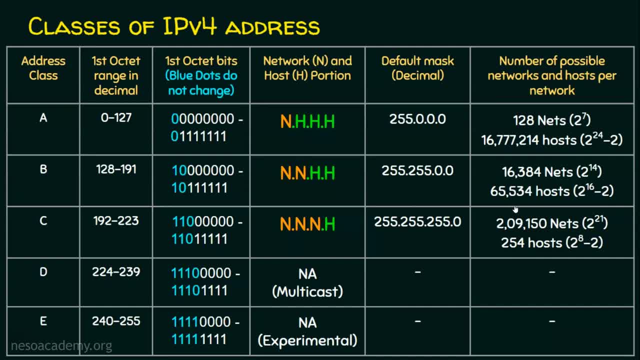 300 devices, we need to go to class B. So in class B we can have a maximum of 65,534 hosts possible per network. In case if our requirement is just 300, no other way, we need to go for class B. 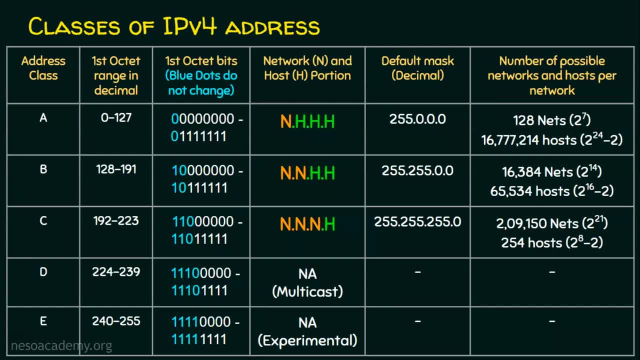 but class B wastes a lot of IP addresses. In the example we have taken we need to create a network with 300 devices or that contains 300 devices. So obviously we can't go for class C, so we need to go to class B. But if we note in class B it can have a maximum of 65,534 hosts or devices, or 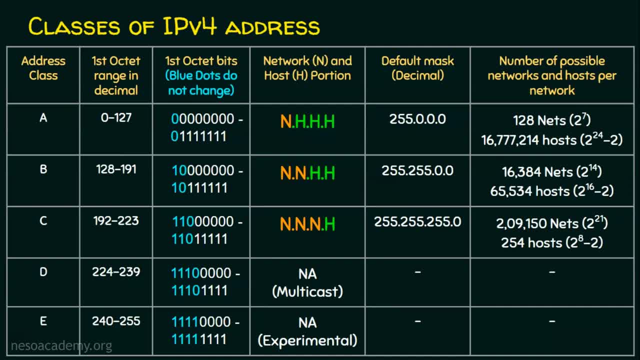 IP addresses, but our requirement is just 300. So 65,534 minus 300 is 65,234 IP addresses. we are going to waste. That's a huge set of IP addresses we are wasting. That's the main drawback of class full addressing In case if we want to have a network which needs. 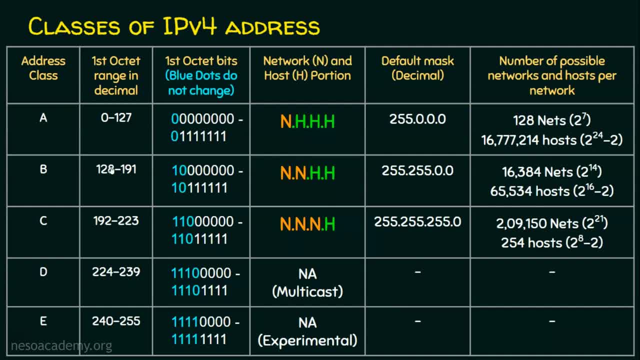 80,000 IP addresses. so obviously we cannot use class B, So we need to go to class A, where class A is a big number of network where it can cater 1,67,77,214 hosts possible per network. So class 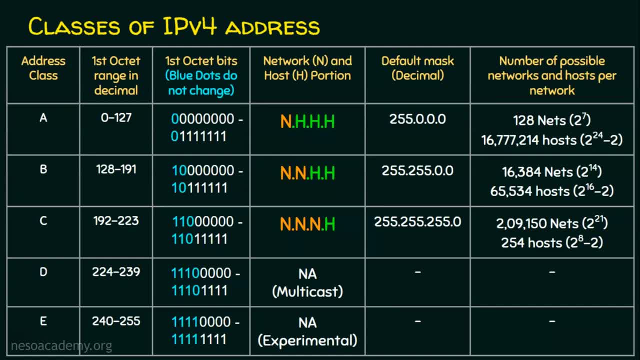 full addressing obviously wastes IP addresses. Say, if I want to create a network that needs only 5 devices, I need to obviously go to class A, where class A is a big number of networks where it can go for class C, Because in a classful world, class C has this many networks wherein in each network, 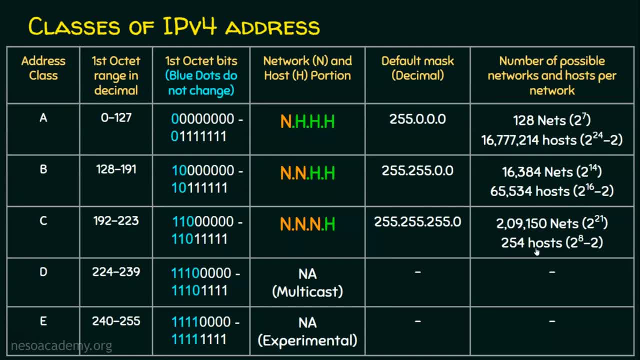 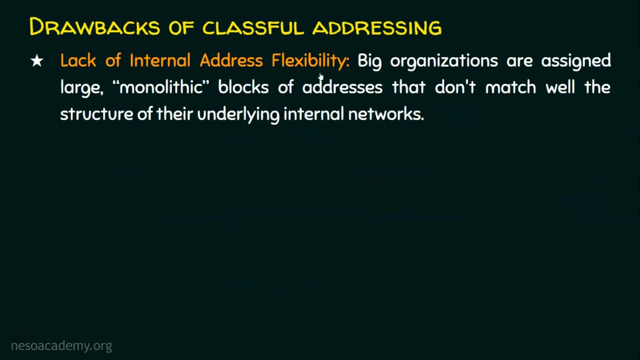 we can have 254 hosts, but our requirement is just 5. So obviously we are going to waste 249 IP addresses. Let's now analyze the drawbacks of classful addressing. Basically, classful addressing has the lack of internal address flexibility. Big organizations are assigned large monolithic 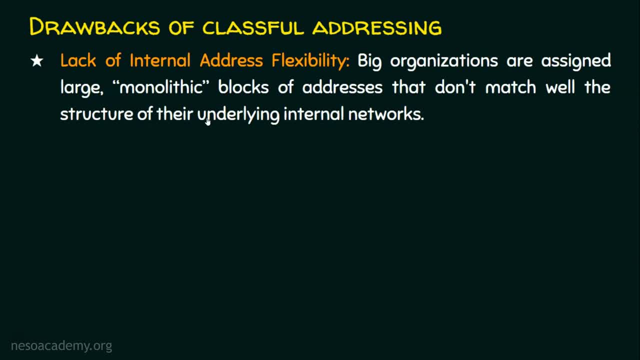 blocks of addresses that don't match well the structure of the underlying internal network. So if we have a big organization, since big organization needs either class B or class C, so these block of addresses that do not exactly match the underlying internal network. 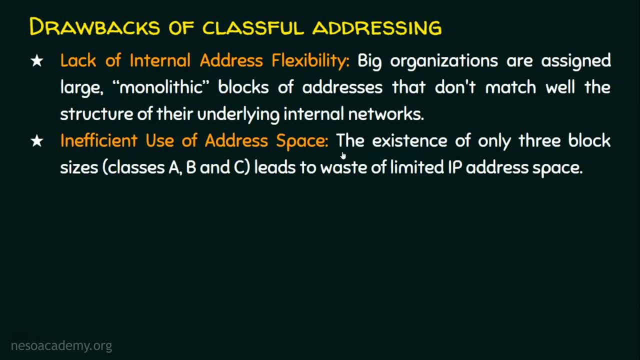 And the second drawback is inefficient use of address space. We know there are five classes of IPv4 addresses and we have only three classes that are used for our general purpose. So the existence of three block sizes may be class B, But these are possibilities within a classless framework. 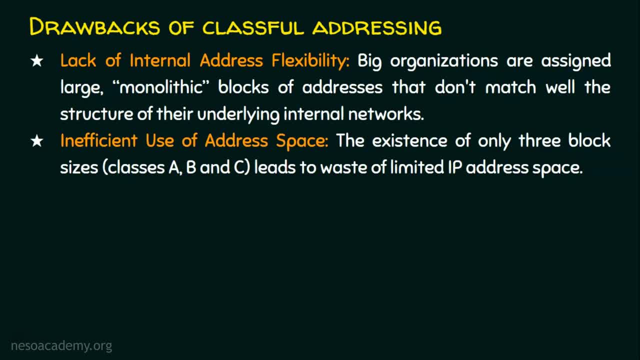 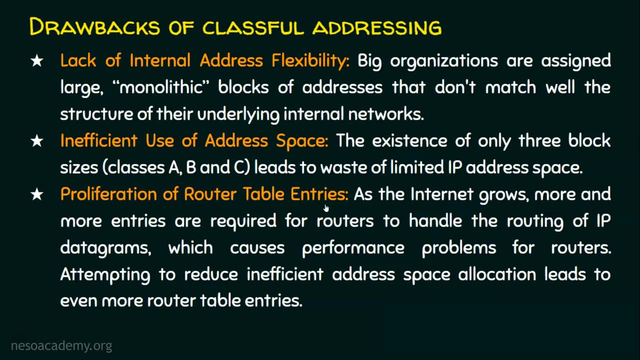 A, class A, B and C lead to waste of limited IP address space. We have already seen this in the previous slide. Classful addressing wastes IP addresses And also the third drawback is proliferation of routing table entries. We know a switch is going to store the MAC address table, whereas a router 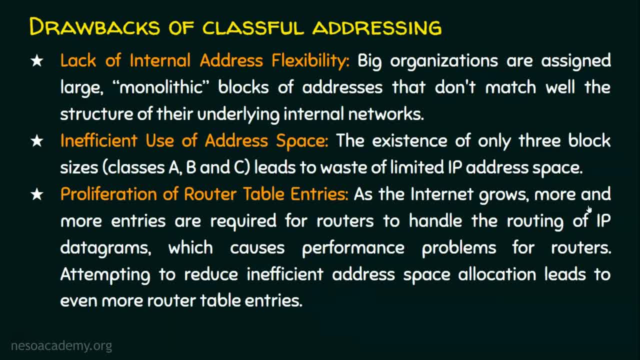 is going to store the routing table. Routing tables are really needed in order to take a decision to required for routers to handle the routing of IP datagrams, which causes performance problems for routers. Attempting to reduce inefficient address space allocation leads to even more routing table entries. 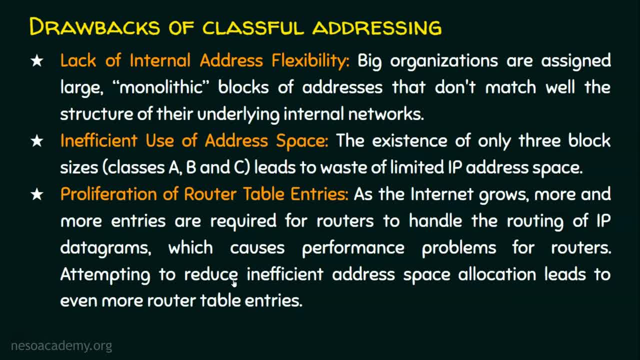 If we take a router, that router is also going to have some memory and this memory is going to store the routing table. In a routing table the IP addresses are going to be stored. What happens if the routing table is a very big one? 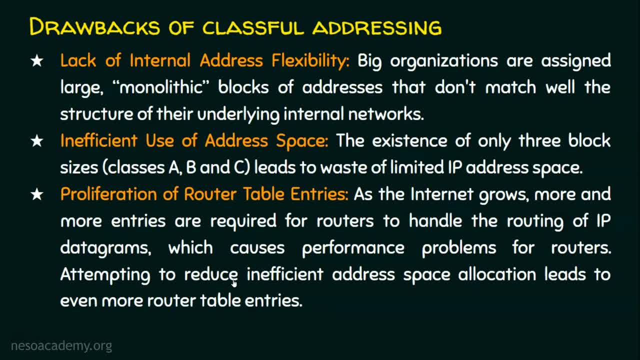 and it's getting increased periodically. Router also has a limited memory size right. It can't handle all IP addresses in the routing table. So when we go for classful addressing, we have this drawback too. So basically, the drawbacks of classful addressing includes: 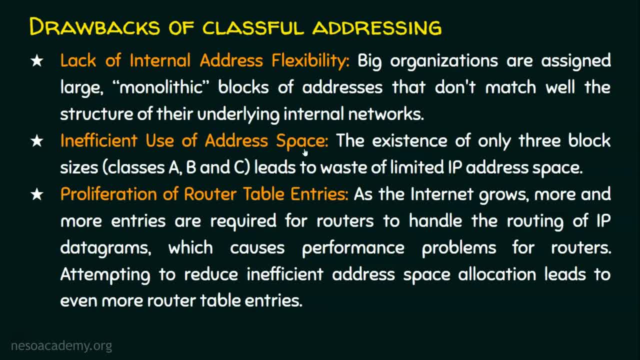 lack of internal address flexibility, inefficient use of address space and the proliferation of router table entries or routing table entries. And because of these problems we need to migrate from classful addressing to classless addressing. In a nutshell, classful addressing wastes IP addresses. 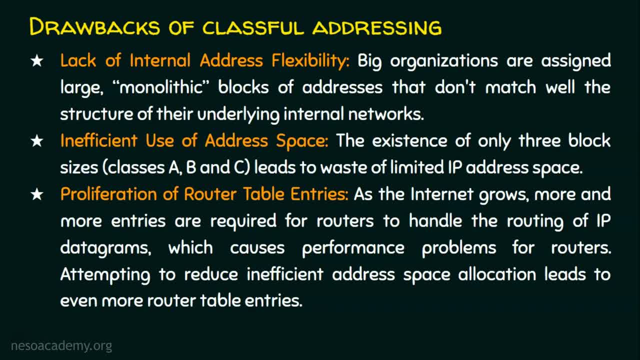 so we need to sparingly use the IP addresses. But with classful addressing, that is, with the fixed subnet mask, it's not possible to save the IP addresses. So that's why we are migrating towards classless addressing. In classless addressing we are going to use the IP address space sparingly.